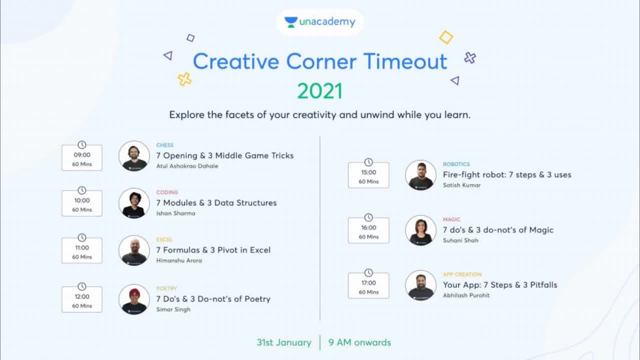 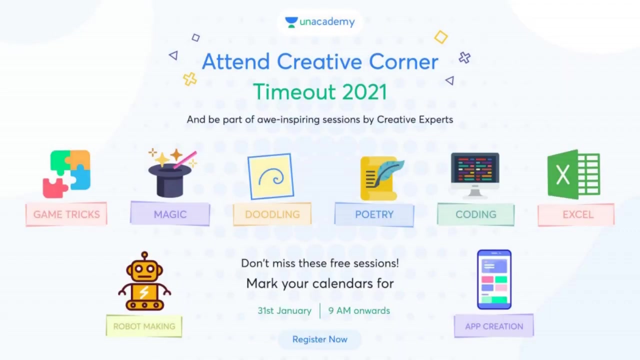 then this is your chance, And the most exciting part is you can win a subscription for Creative Corner by submitting a video, A video of yourself recreating something that you learnt in timeout sessions. So mark the date. be ready to discover the world of creativity and learn new skills. 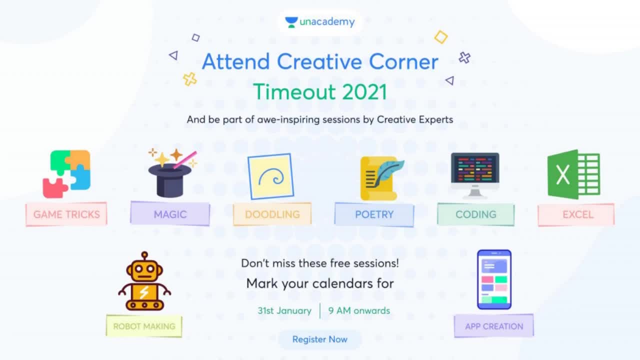 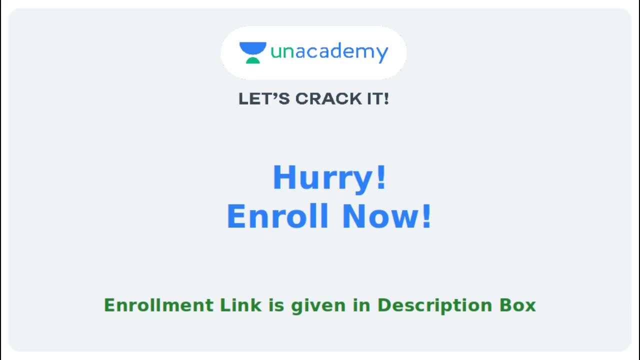 Creative Corner. Timeout is on 31st January 2021.. Sounds interesting. To enrol free for this event, you need to check the enrolment link given in the description box To enrol. you can also download the Unacademy app from the Play Store. 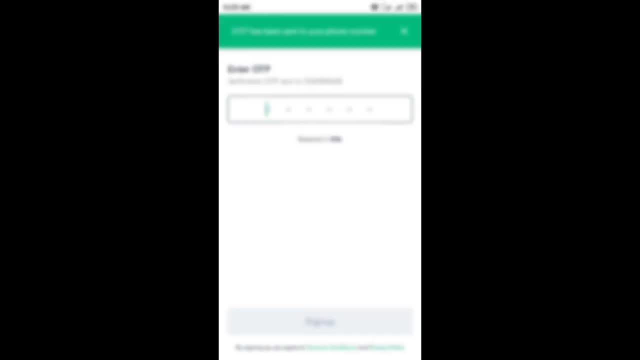 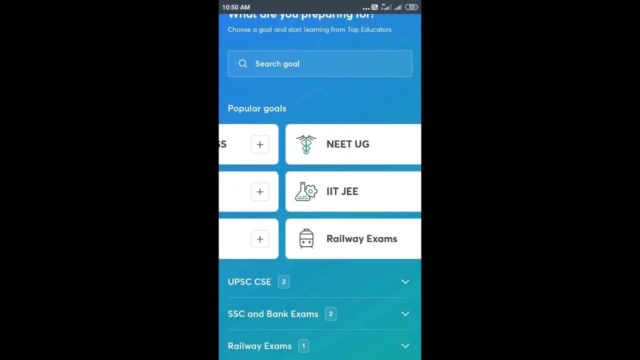 Then enter your mobile number for sign up. Fill all the details, such as your name, email address and your state. By completing this process, you will get an OTP on your mobile number. Just enter the OTP and you will be in Unacademy family. 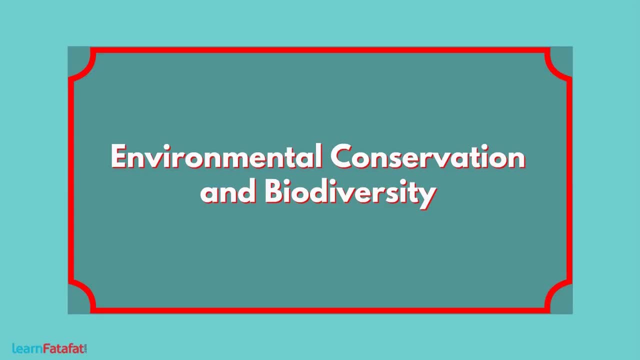 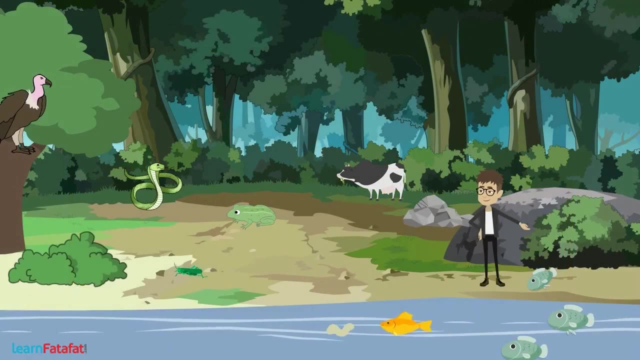 So let's crack it: Environmental Conservation and Biodiversity. Everything around us is called environment. It includes living and non-living things and the interrelationship between living and non-living things and the interrelationship between living and non-living things. 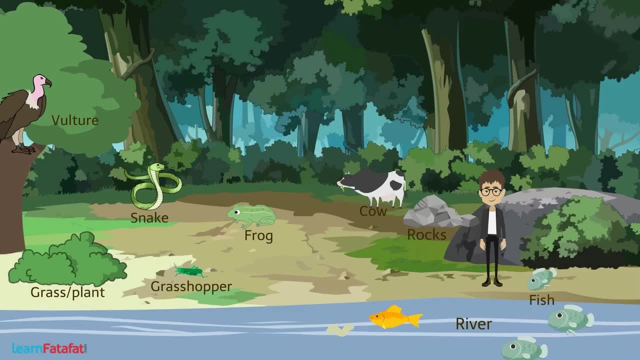 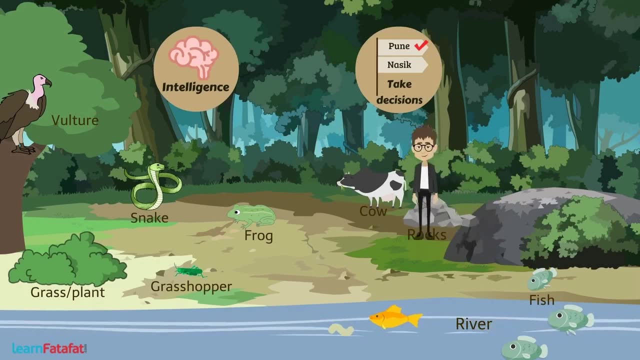 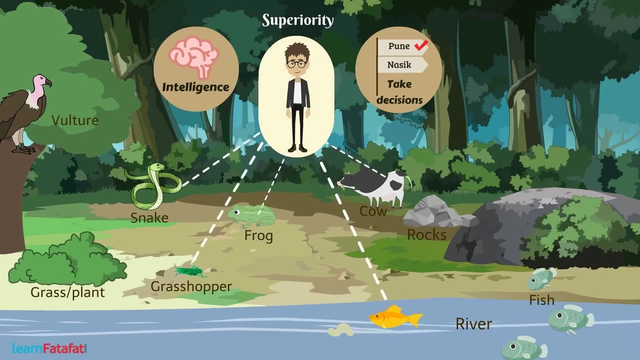 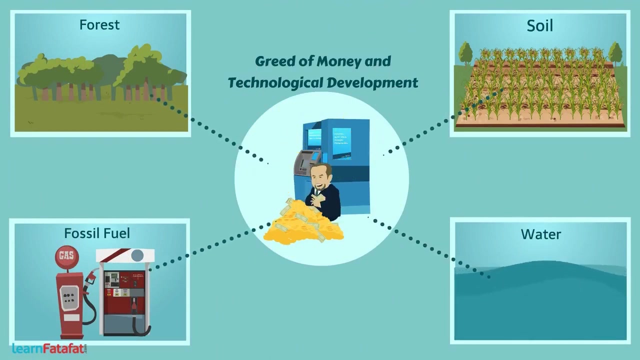 among them, There are millions of organisms living on earth with characters like intelligence, ability to take decisions, etc. Human being has proved his superiority and established domination over all others. For the greed of money and technological development, he started using the resources as much as he can. 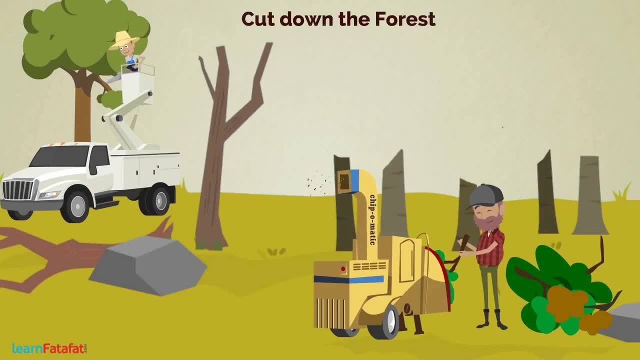 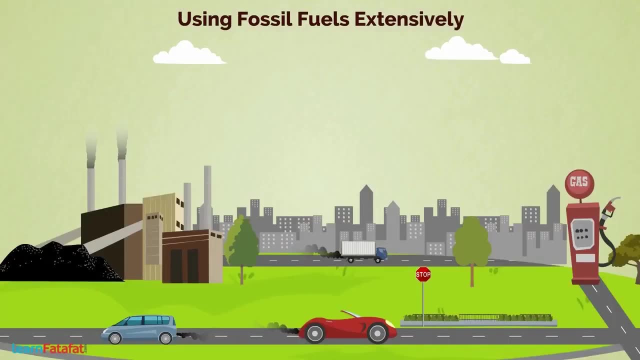 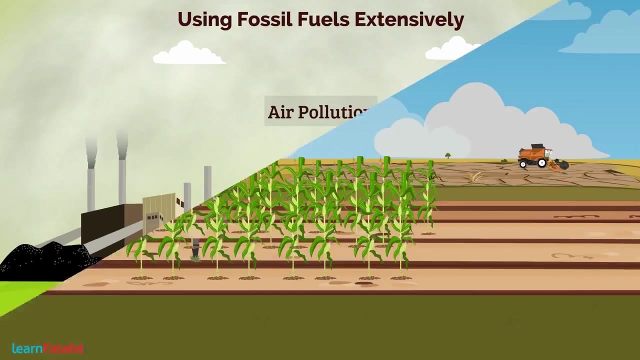 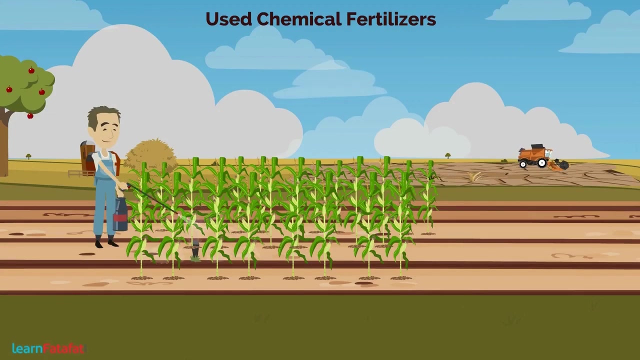 Human being never cared for the nature. he cut down the forest, thereby destroying the habitat of many organisms. He kept on using fossil fuels extensively, which caused air pollution. For getting better agricultural output, he used chemical fertilizers and other chemicals, which caused soil pollution. 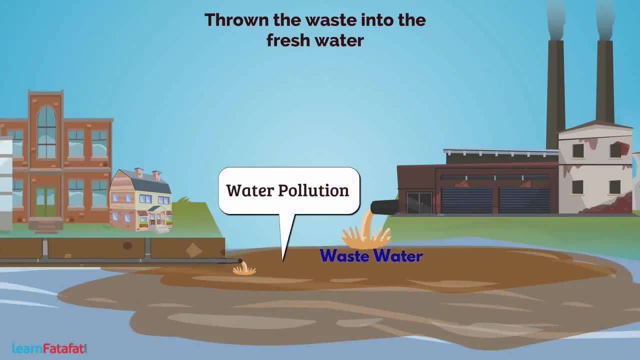 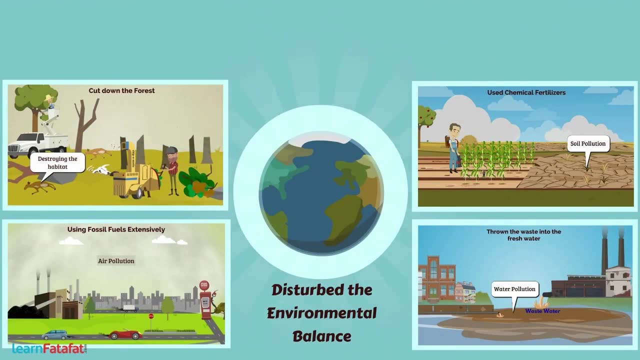 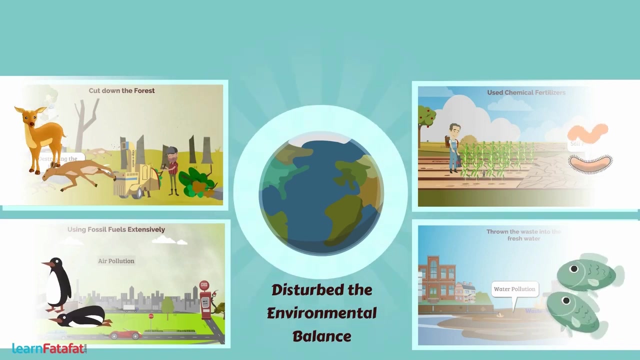 He throwed the waste into the water and threw it into the soil. He threw the waste into the fresh water bodies and polluted water. All these activities disturbed the environmental balance. The habitat of many organisms have been destroyed, which affected the survival of those species. Many species became extinct and many are on the verge of extinction General. 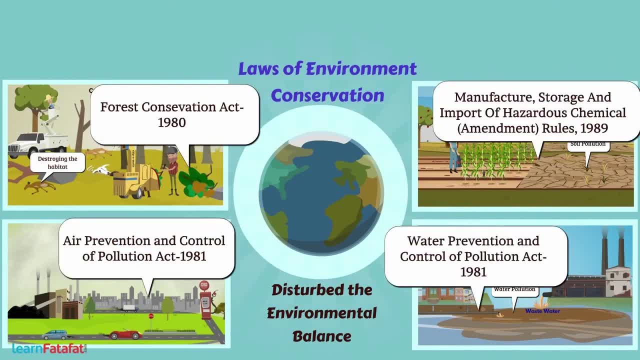 public, including us, is not aware about the laws and regulations of environment conservation. Even if we know, still, knowingly or unknowingly, we neglect them. There is a need of large scale participation of people for conserving our environment. Environmental conservation deals with the protection, preservation and restoration. 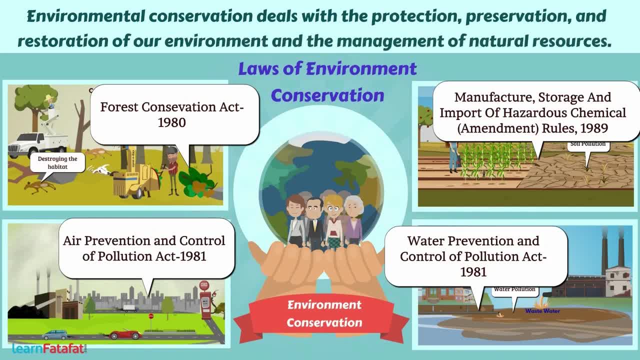 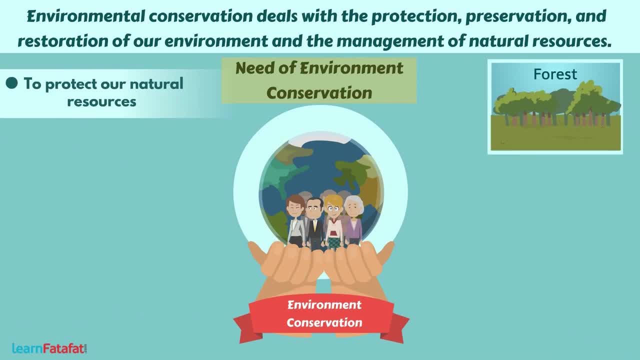 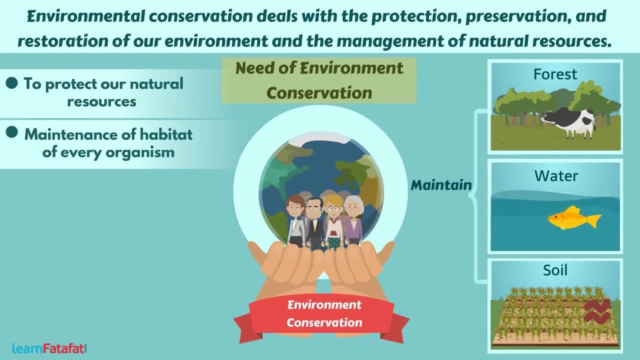 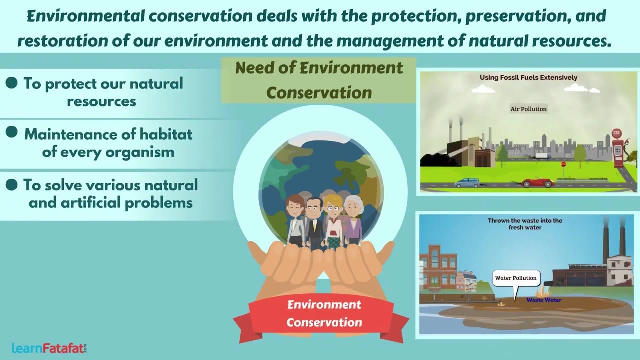 of our environment and management of natural resources. Environmental conservation is needed to protect our natural resources like forest, water, soil, etc. It is needed for the maintenance of habitat of every organism on earth and for survival of species on the earth. It is needed to solve various natural and artificial problems. It is 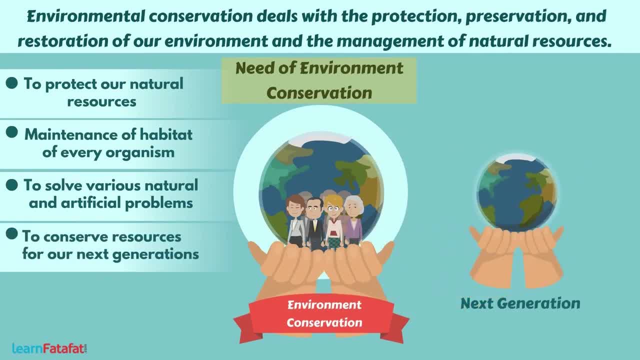 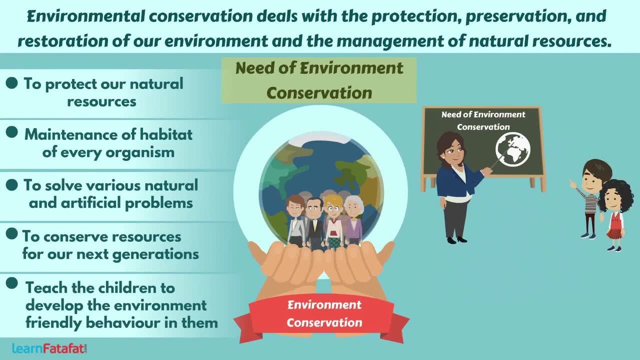 needed to conserve resources for our next generation. It is needed to maintain the balance in nature. The teachers- parents- should teach the children about it and develop the environment friendly behavior in them. It will help our future generation to become aware of environmental problems and thus they can give a helping hand for conserving our environment. Today, all countries 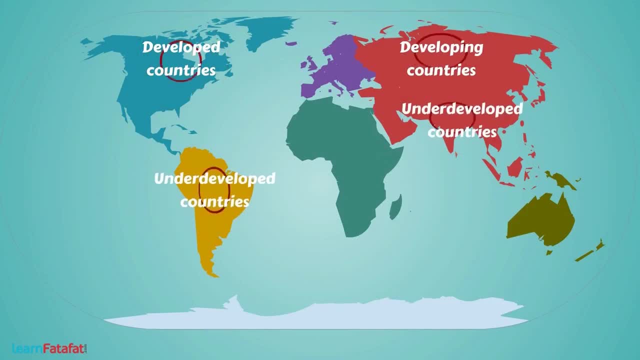 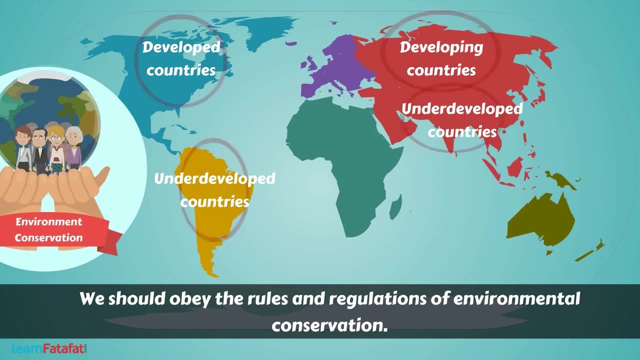 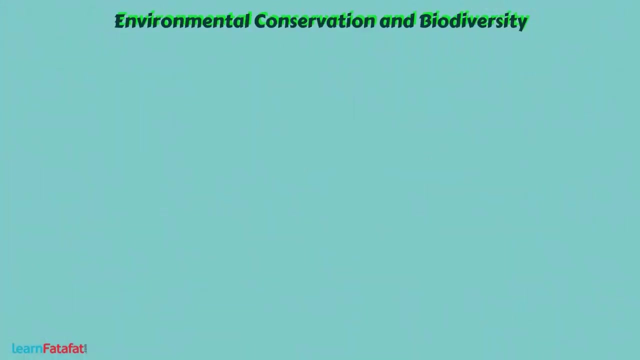 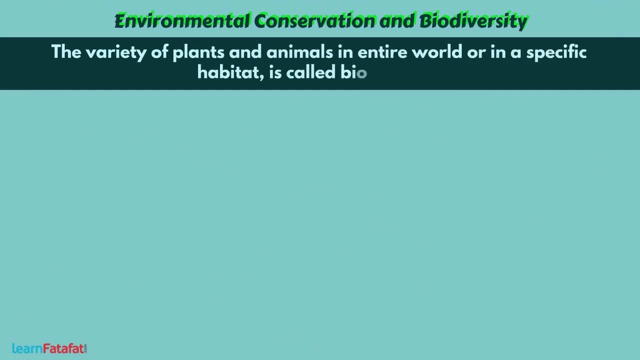 including developed countries, developing countries and underdeveloped countries, have taken the responsibility to conserve the environment. We should obey the rules and regulations of environmental conservation, Environmental Environmental conservation and biodiversity. The variety of plants and animals in entire world or in specific habitat is called biodiversity. Biodiversity occurs at different levels: Genetic biodiversity. 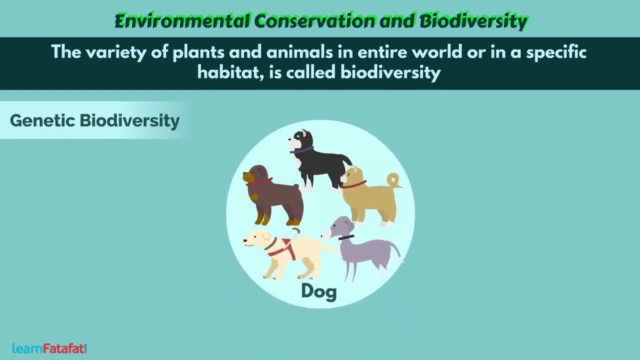 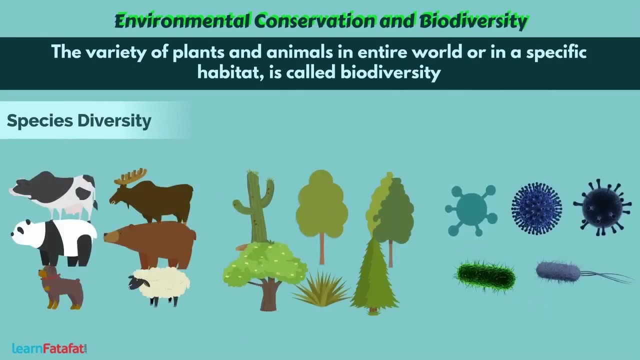 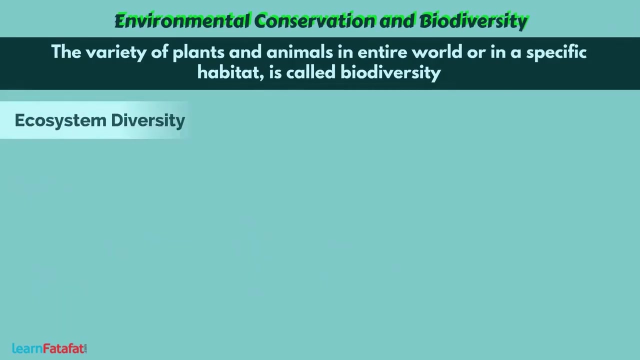 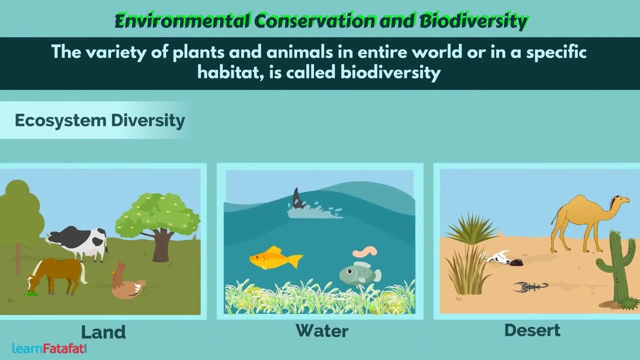 The diversity among the organisms in a same species is called genetic biodiversity. If the genetic diversity decreases, the possibility of survival of that species also decreases. Species diversity: There are different species in the living world, which includes species of animals, plants andA 50%.